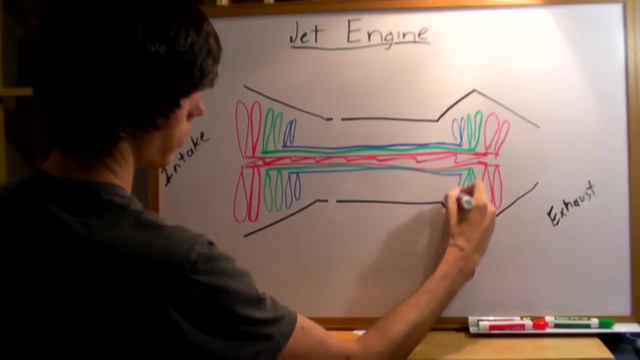 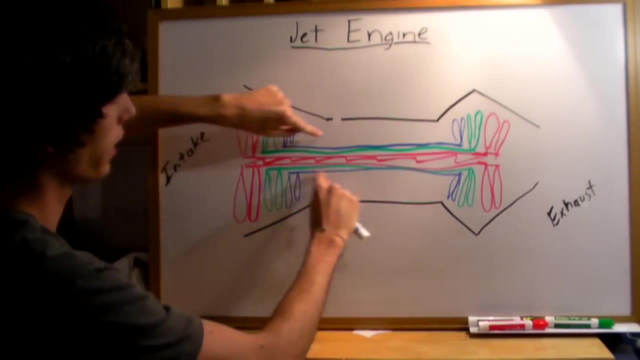 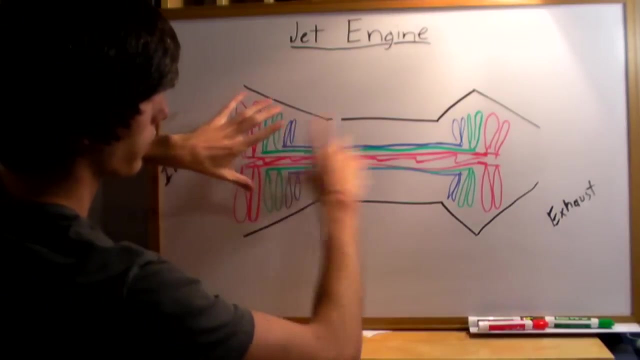 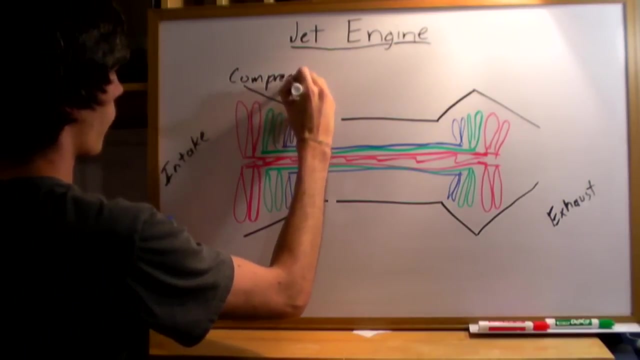 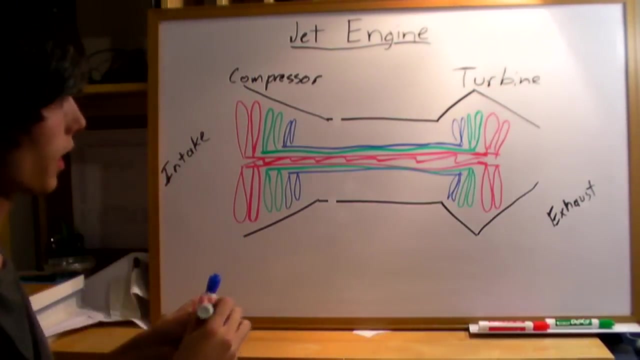 So, as you can see, what's happening here is: this will be rotating on the inside and then inside of that, this green shaft will be rotating with both the turbine, with the compressor, over here in the turbine. go ahead and label that so we've got our compressor and we've got our turbine, and so what's going to happen is. 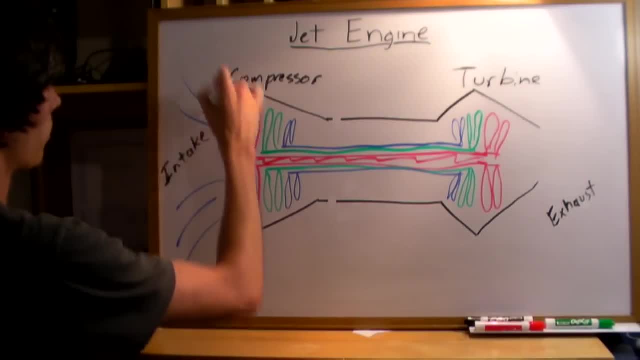 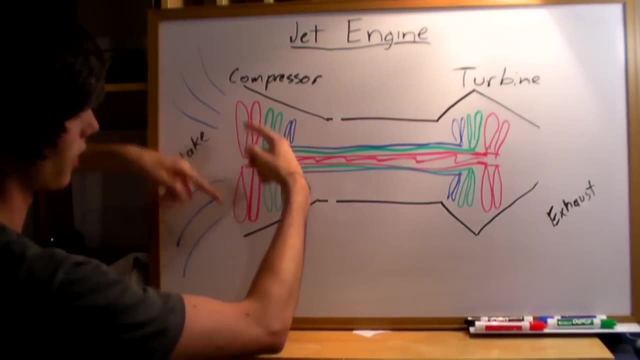 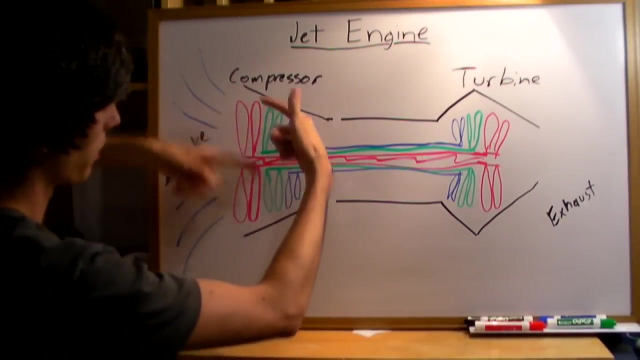 air is going to flow into this compressor and as that air flows in, this first shaft is going to be rotating the slowest and it's going to squeeze the air in, and then this second shaft will be rotating a bit faster and it's going to squeeze it more, and so the air is going to accelerate the entire time it's. 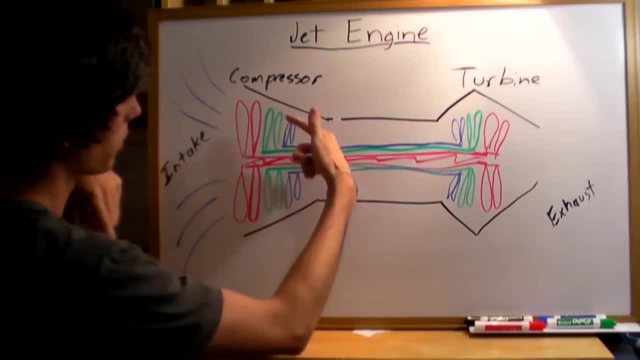 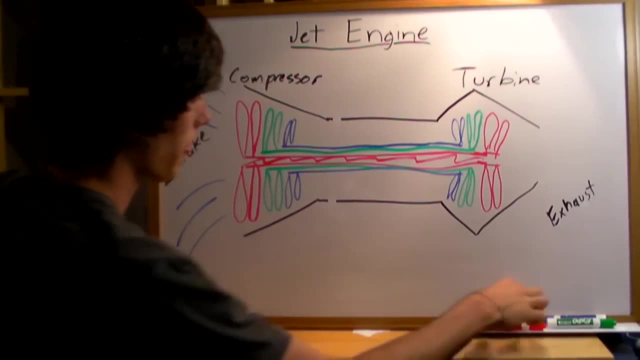 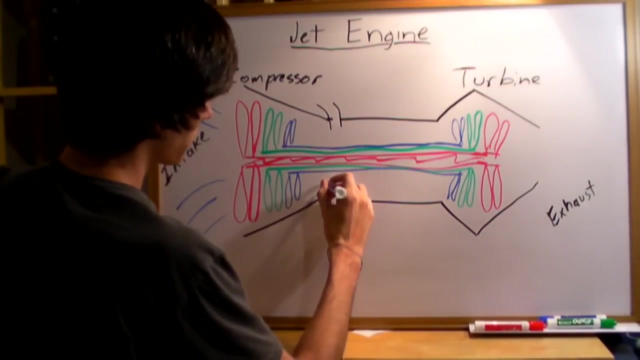 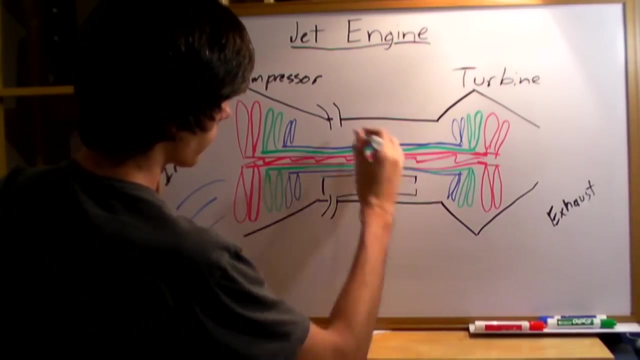 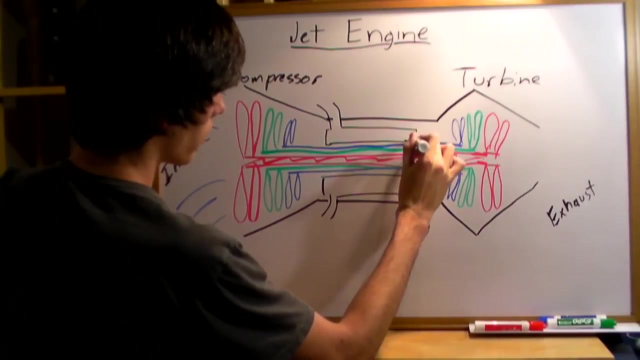 moving in. finally, when it gets to this blue shaft, it's going to be rotating extremely quickly and still compressing it further. so it's getting smaller and moving faster. That's the goal. Then we're gonna get into the combustor And there's going to be a bunch of these combustor cylinders moving around. 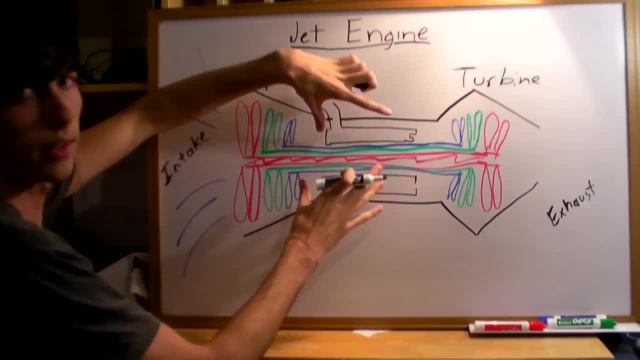 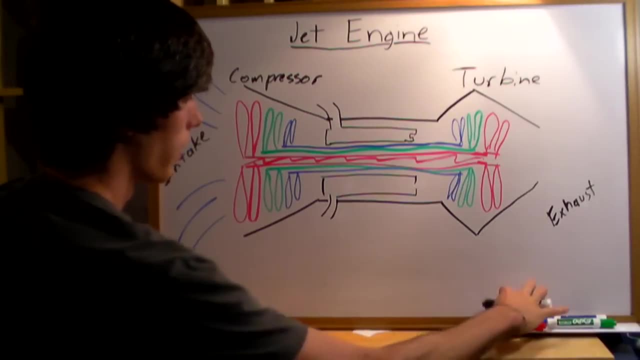 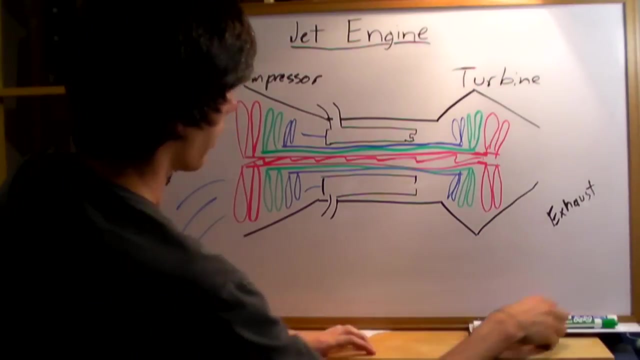 rotating. They stay in their place, but they're gonna be placed around these shafts. these shafts are going to rotate inside of them, So this air is going to be forced in to these combustor chambers And fuel is going to be supplied into them, and then you'll have an igniter inside of the. 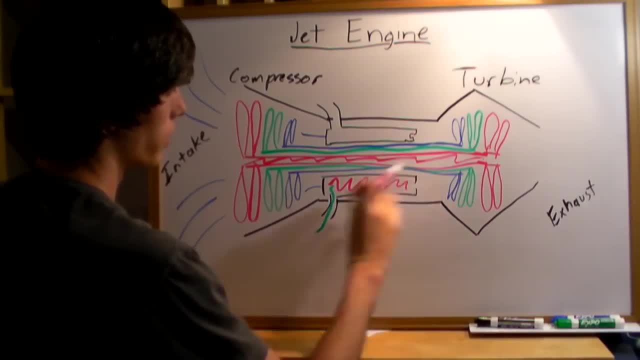 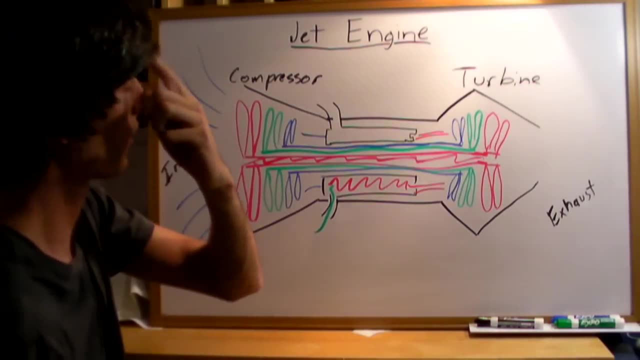 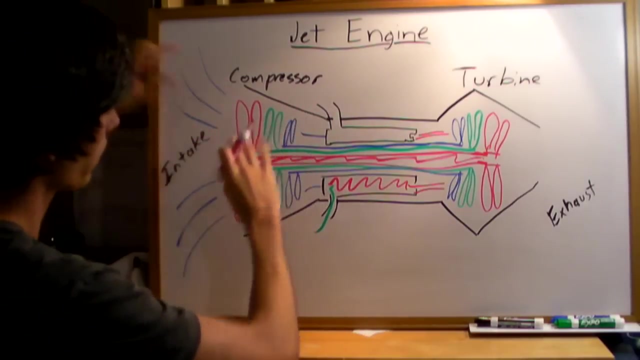 combustor, so that creates the combustion, So it explodes, expands, it's like the air that's flowing out. Huh, and then it forces that hot air into the turbine. Now the turbine. some of that air will go into rotating these compressor fans over here and sucking in air. 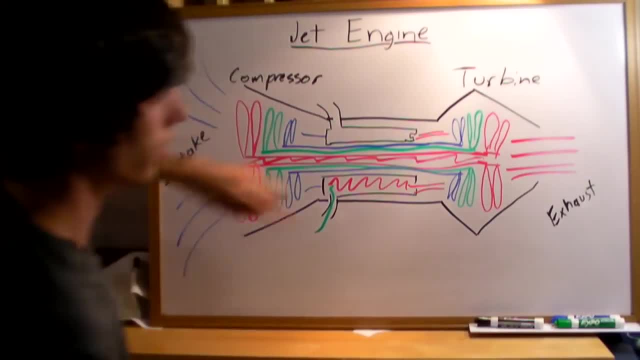 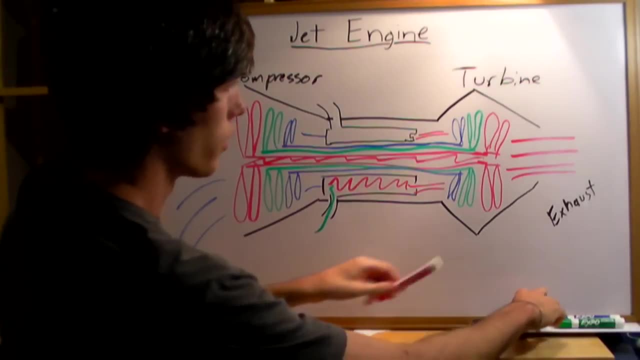 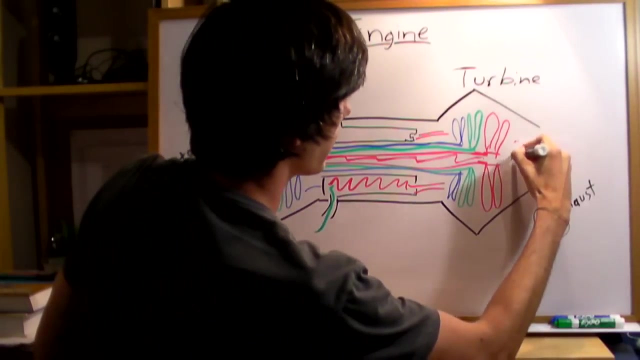 The rest of it will be forced out the back at a very high rate, much quicker than the air is being pulled in, and so it will provide a forward thrust. Now, other things you can do with it is: you can attach a blade. put a blade right here.